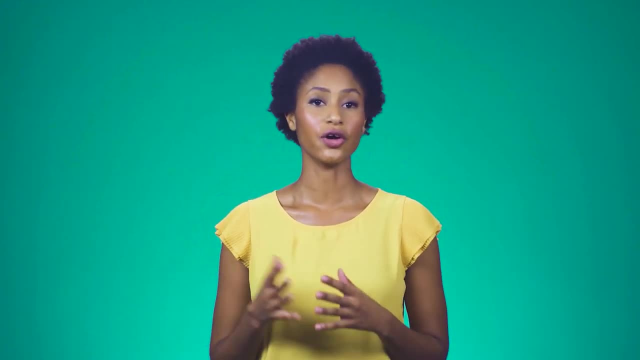 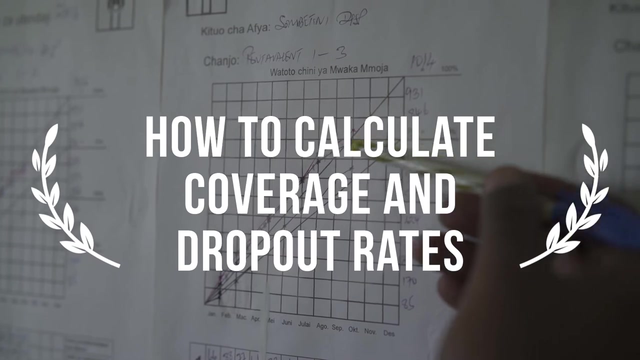 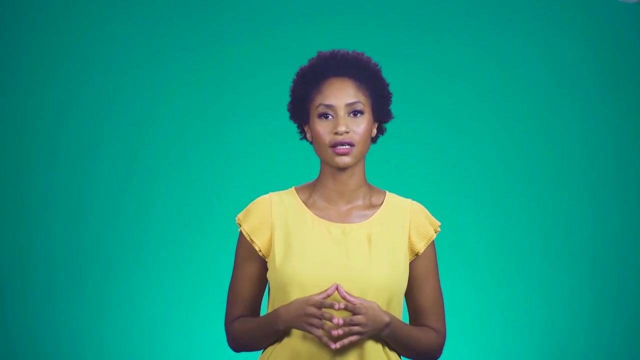 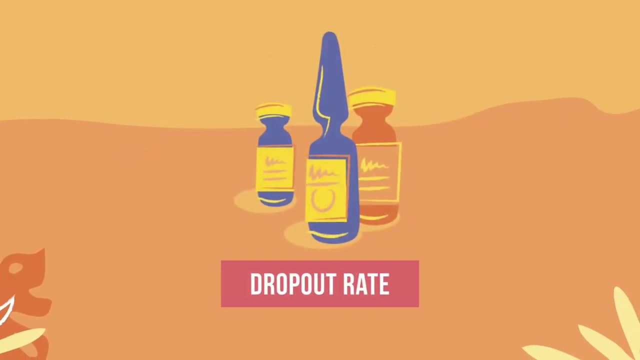 Two of the most important pieces of data for you to know are your coverage rate and your dropout rate. The coverage rate shows the percentage of your target population that has been immunized with a particular dose of a vaccine. The dropout rate shows the percentage of infants who started. 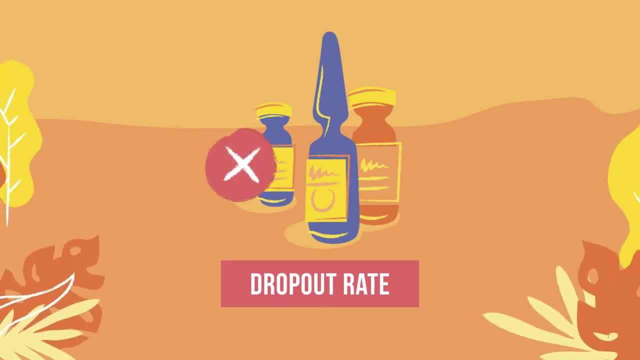 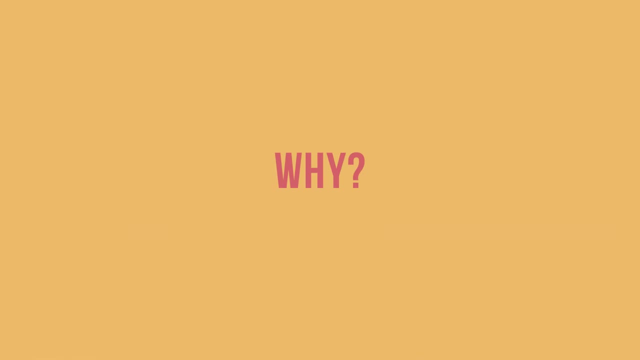 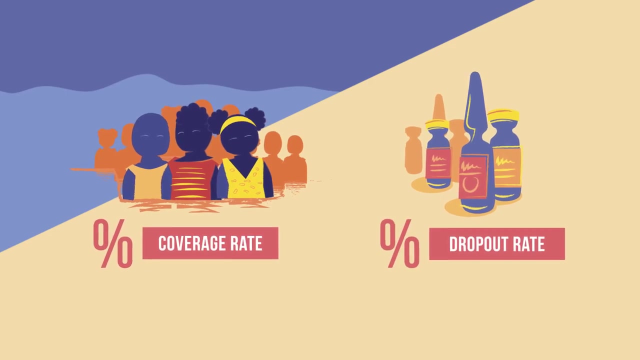 receiving immunizations but never received all doses in a series. Calculating these two numbers is something you should do every month. Why should you do it? Because both of these pieces of data will help you discover potential coverage problems Once you have discovered a coverage. 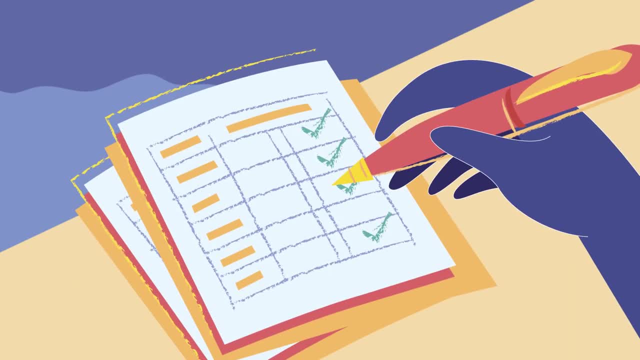 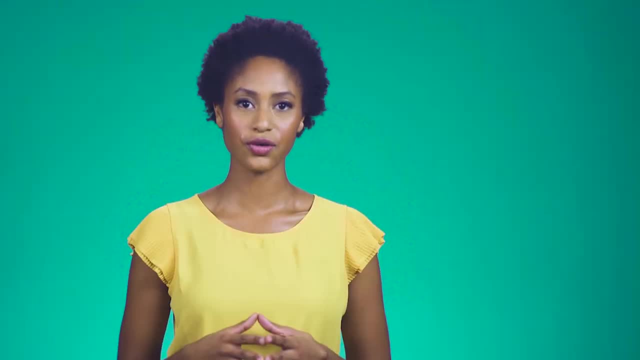 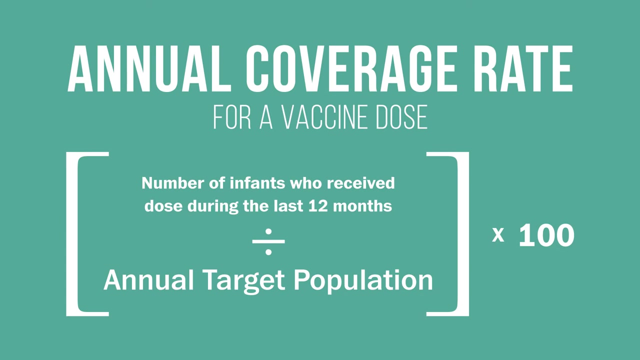 problem. you can figure out what sort of action you should take to increase your coverage. Let us look at how you calculate each of these numbers, starting with the coverage rate. Here is the formula for calculating your annual coverage rate. We are going to work through this formula step by step. 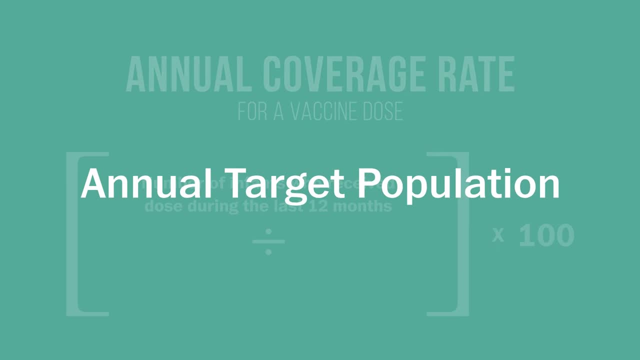 First write down the annual target population for the community. The target population may be the number of infants under one year old or pregnant women. Use the official data given to you by the Ministry of Health and Human Services. If you have any questions, please contact the Ministry of Health and Human Services. 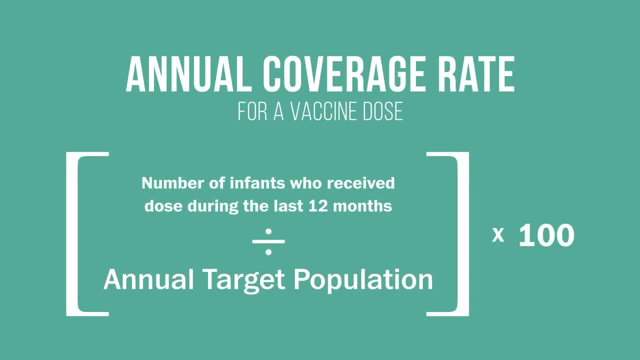 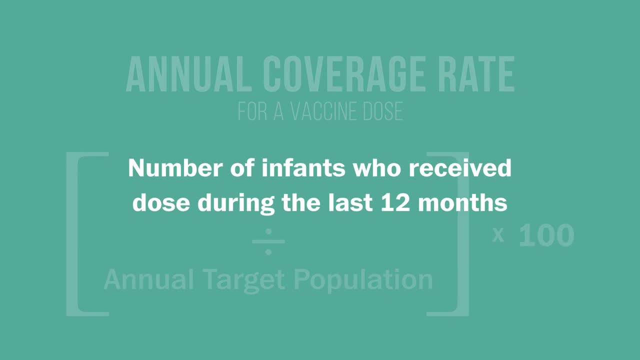 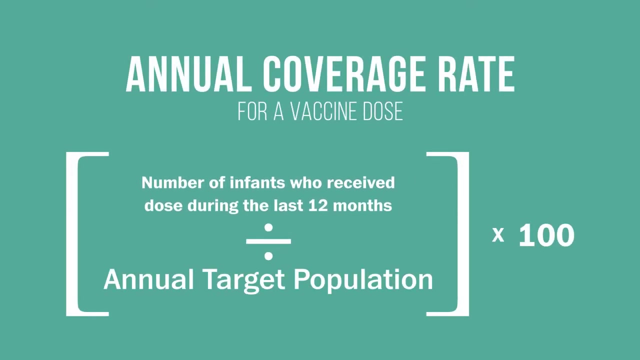 Next, for a particular vaccine type or a specific dose of that vaccine, tally the total number of doses you delivered during the preceding 12 months, Now divide the number of doses delivered by the annual target population and multiply that number by 100. The result is the coverage rate for the particular vaccine dose.